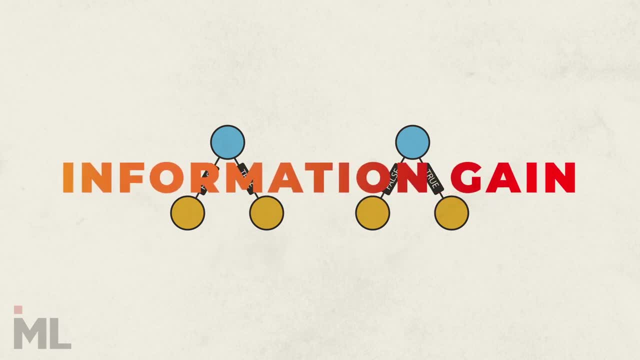 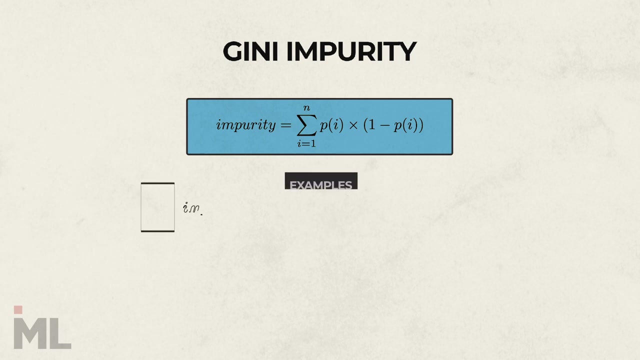 centerpiece of this step. So what is information gain? Let's have a closer look at each group within a decision rule. The group is pure when all of its records belong to the same class. Here we use gaining impurity to measure how pure the current node is When the group is pure. 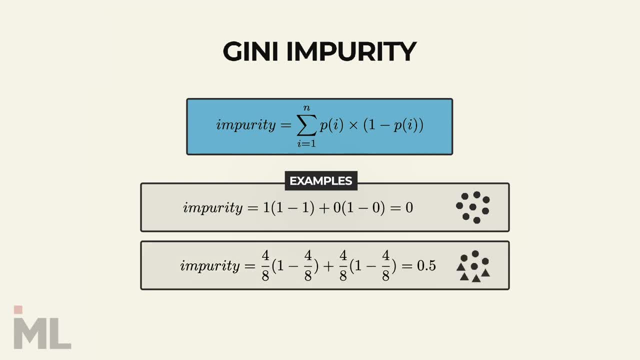 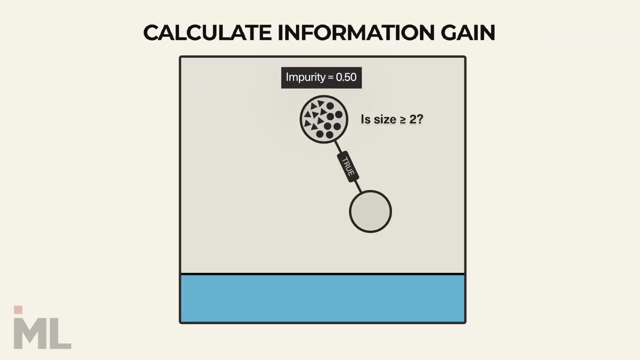 gaining impurity is 0.. When the group is half and half mixed, gaining impurity is 0.5.. For any decision split, a parent group is split into two child groups. The information gain of this split is the impurity of the parent group. 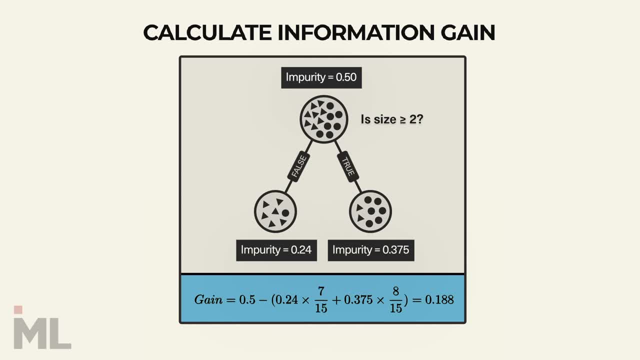 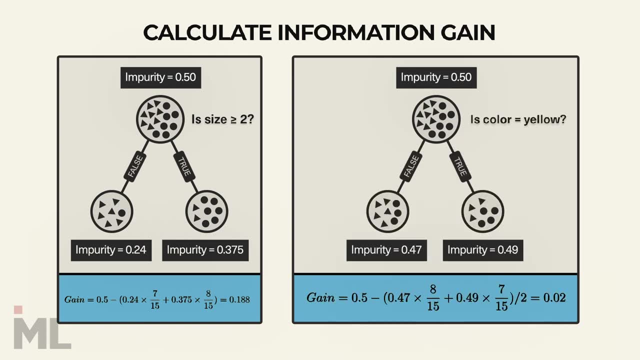 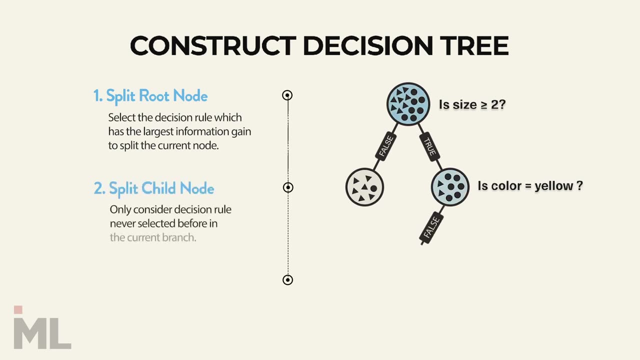 minus weighted average. impurity of the child group. Once we calculate the information gain of each splitting decision rule, we now can select the decision rule which has the largest information gain to split the current node. Then we can split the child node recursively and only considering decision rule never selected before in the current branch. 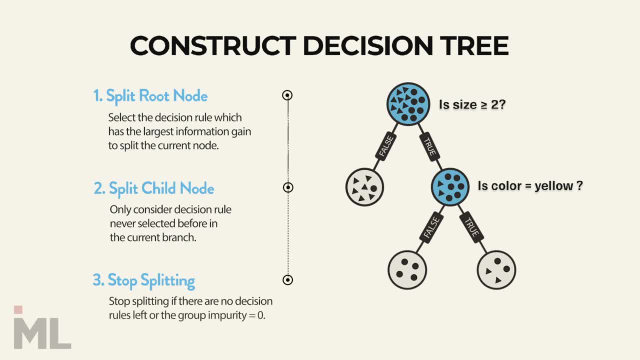 We stop splitting if there are no decision rules left or the group impurity is 0. Sometimes pruning and early stop condition are used to prevent a large number of splits and overfitting. Now the decision tree can predict the probability of each class at the 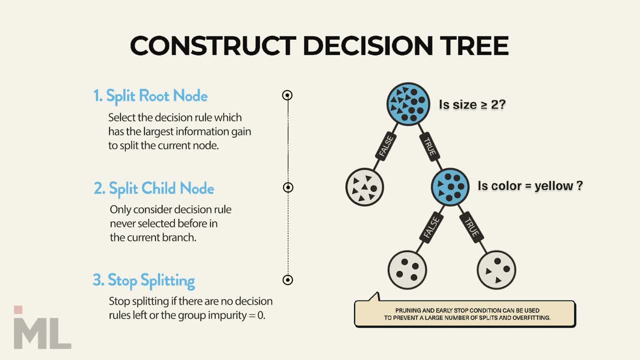 ratio of each class in the node. In this case, for the record which says greater or equal to 2 and color is yellow, there is a 50% chance. the class record is a circle, So that is a brief demonstration of how to construct a decision tree from data. 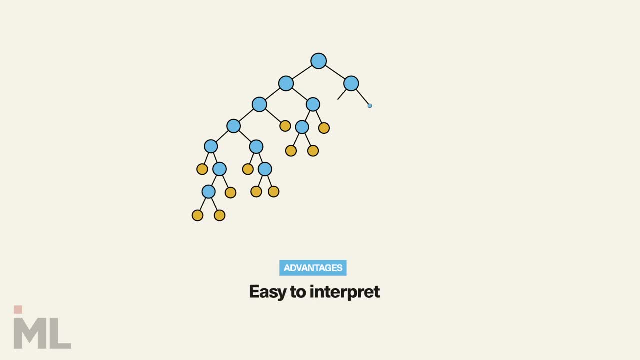 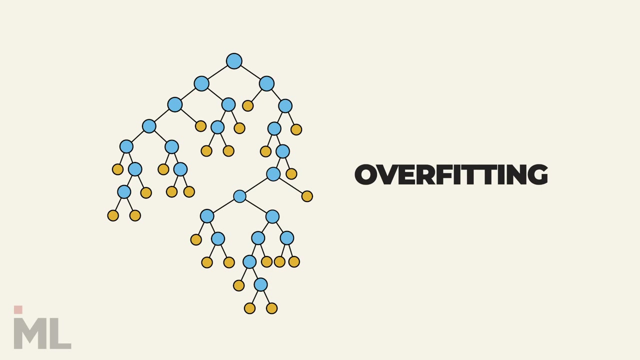 It has a lot of advantages, Like easy to interpret and straightforward for visualizations. However, it has a big disadvantage: Single decision. tree models are prone to overfitting, especially when a tree is particularly steep. One way to combat this issue is by setting a max depth of the tree. 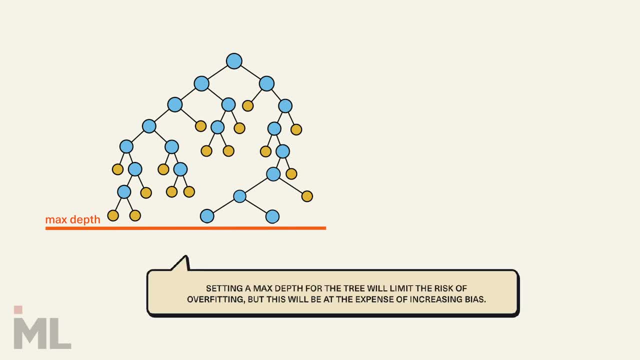 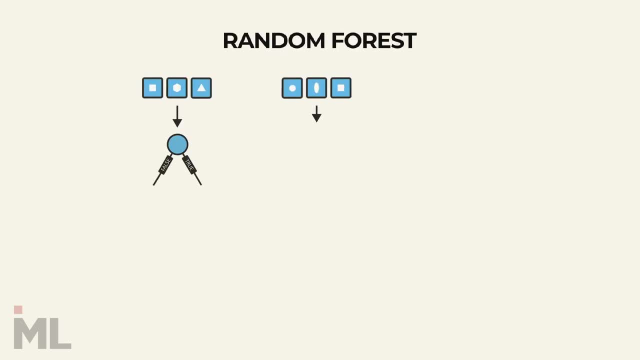 This will limit the risk of overfitting, but this will be at the expense of increasing bias. Random forest is a good way to prevent overfitting. It is simply a collection of decision trees whose results are aggregated into one final result. It is a strong ensemble modeling technique and much more robust than a single decision tree.